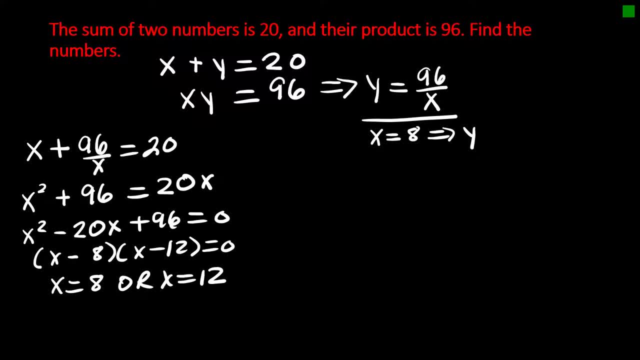 If X is 8,, then Y is going to be 96 divided by 8,, which is 12.. And if X is 12,, Y is going to be 96 divided by 12,, which is 8.. So in either situation, 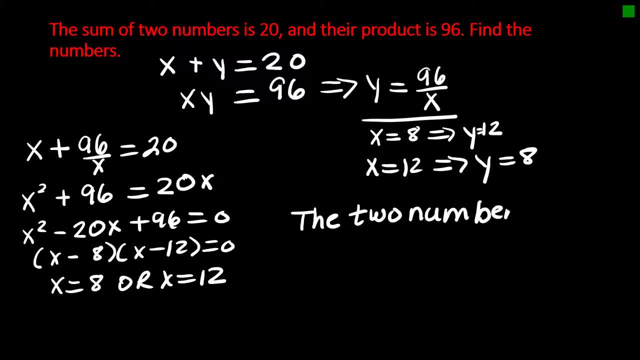 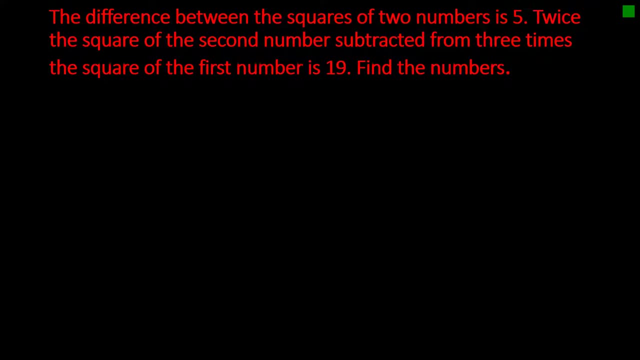 the two numbers are 8 and 12.. Let's look at another one. The difference between the squares of two numbers is 5.. Twice the difference, excuse me, twice the square of the second number is subtracted from three times the square of the first number, and that is 19.. 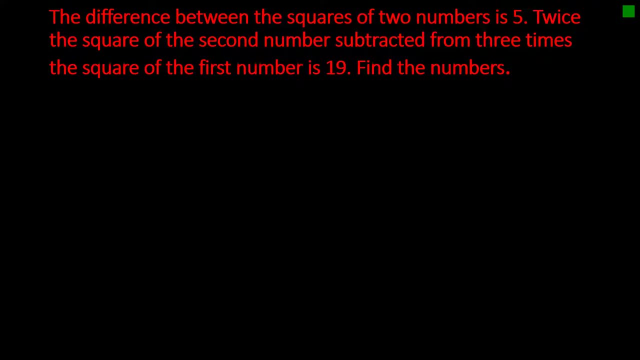 Find the two numbers. So the difference between the squares of two numbers is 5.. So if I have a number X and a number Y and I square it and I take the difference, that result is 5.. Two times the square of the second number. 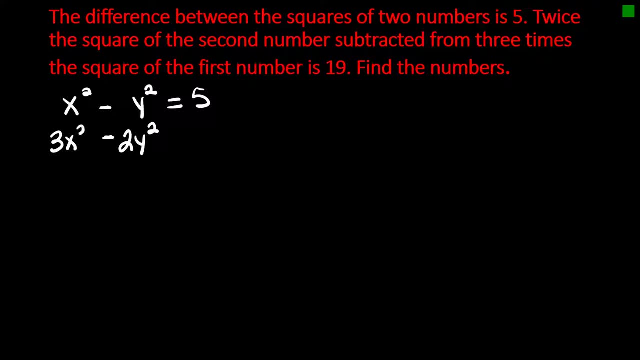 subtracted from three times the square of the second number, three times the square of the first number, is 19, and let's find these numbers. well, um, I can use elimination here. I can multiply my first equation by negative 2 and I can eliminate the Y's, so I have negative 2x squared plus 2y. 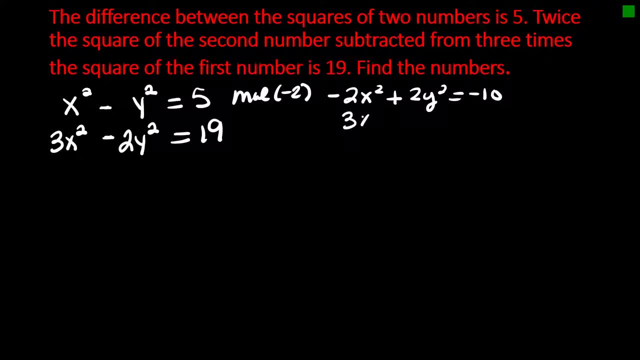 squared equals negative 10. my first, excuse me, my second equation stays the same. when I add, I get x squared equals 9. so X is going to be plus or minus 3. so now I need to find y and I'm gonna go here and I'm gonna solve for y, y squared.